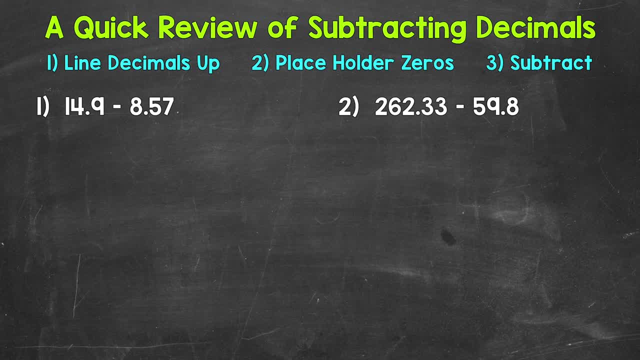 really no matter what class or goal you are working towards. here are a couple of examples to get this down. Let's jump into number 1, where we have 14 and 9 tenths minus 8 and 57 hundredths. 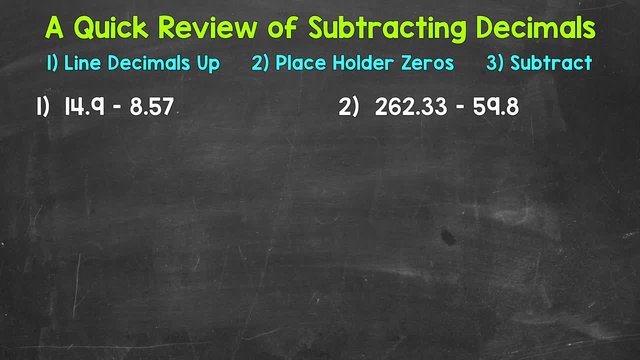 Now, just like when we add decimals, when we subtract decimals, we need to line the decimals up. That's going to line up all of our places. So let's rewrite this first problem vertically here, lining up the decimals. So 14 and 9 tenths minus 8 and 57.. 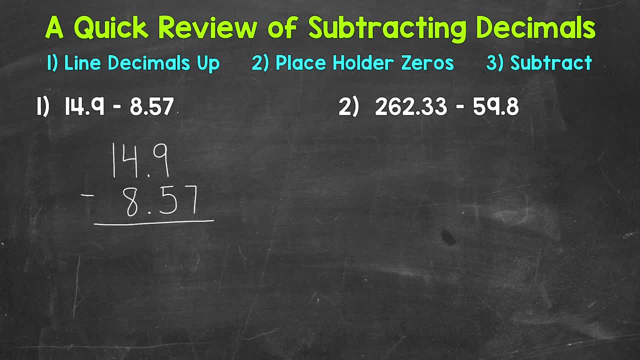 So the decimals are lined up and that's going to line up all of our places. Now that problem looks a little offset, because 14 and 9 tenths goes to the tenths place and then 8 and 57 hundredths goes to the hundredths place. 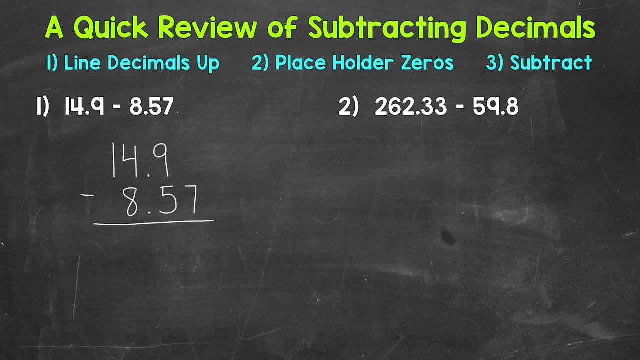 So, just like when we add decimals, we can use placeholder zeros to have this look more lined up. So let's use a placeholder zero in the hundredths place here and then both of our decimals go to the hundredths place. Remember, zeros to the right of a decimal do not change the value. 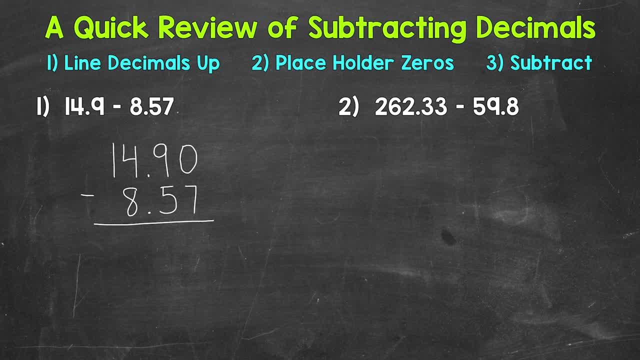 That's an equivalent decimal and does not change the value of the problem at all. Now we're able to subtract, So we'll start with the hundredths place. We have 0 minus 7, which we need to borrow, So let's borrow from the 9.. 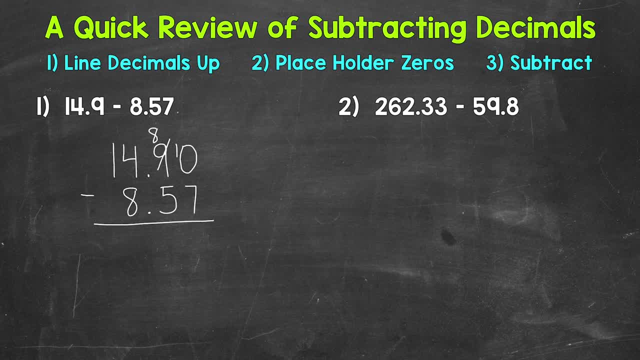 That's an 8 now, And we have 10 minus 7, which is 3.. Then we move on. We move to the tenths place: 8 minus 5, 3.. Bring our decimal straight down into the answer. 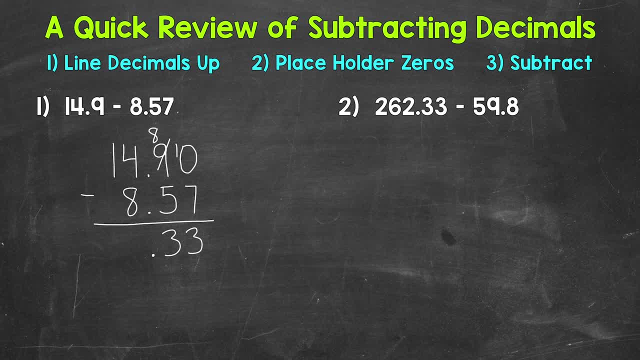 The decimal is lined up throughout the entire problem. Then we move to the ones place, 4 minus 8.. We need to borrow from the tens place here. So that's a 0, and that's a 14.. So 14 minus 8 is 6, and we are done. 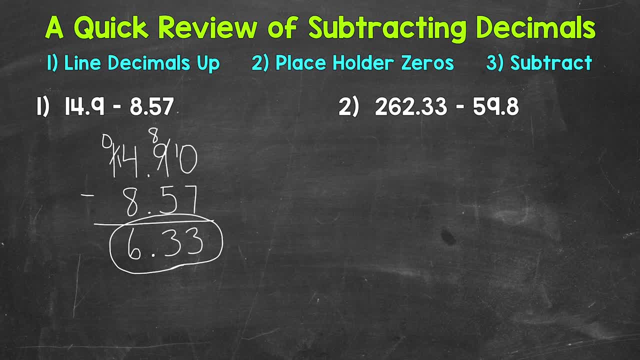 6 and 33 hundredths. Now I do want to mention one more thing before moving on to number two, And this is going to be a common mistake that you'll want to avoid, And using placeholder zeros will actually help you avoid this mistake. 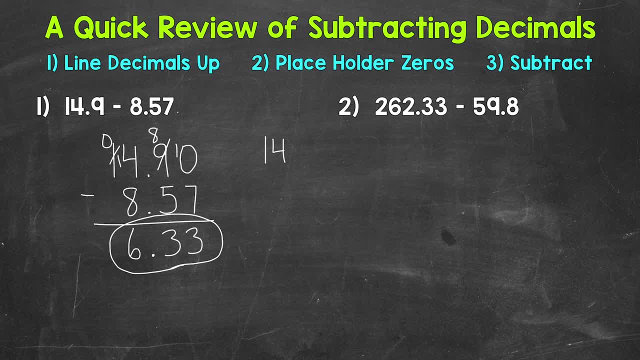 So let me rewrite the problem here real quick, to the side. So we have 14 and 9 tenths minus 8 and 57 hundredths, So dropping this 7, so starting with the hundredths place and then just dropping the 7 because there isn't anything above, it is not correct. 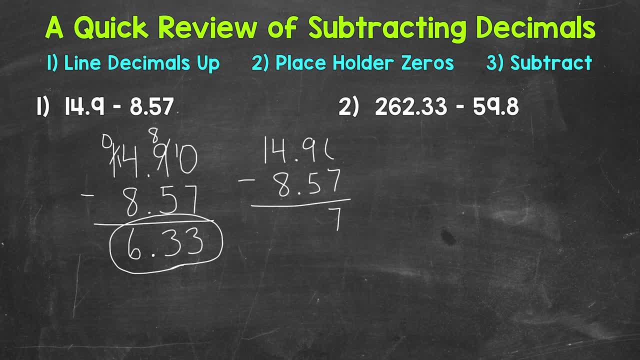 We actually have 0 minus 7 there, so we needed to borrow And you can see we do not have a 7 in the hundredths place in our final answer. So again, avoid the mistake of just dropping that number, because really we have 0 minus 7 there and we need to borrow. 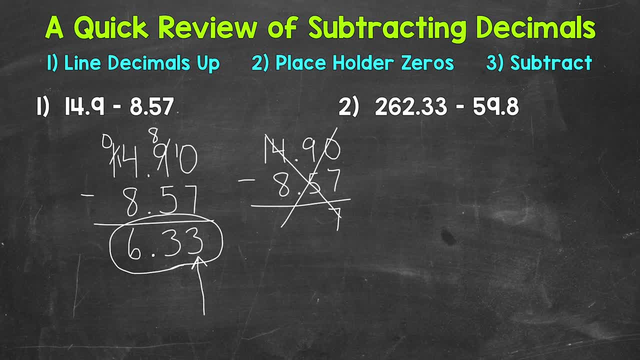 So be careful of that. Let's move on to number two, where we have 262 and 33 hundredths minus 59 and 8 tenths. So we will start by lining up our decimals here, So 262 and 33 hundredths minus 59 and 8 tenths. 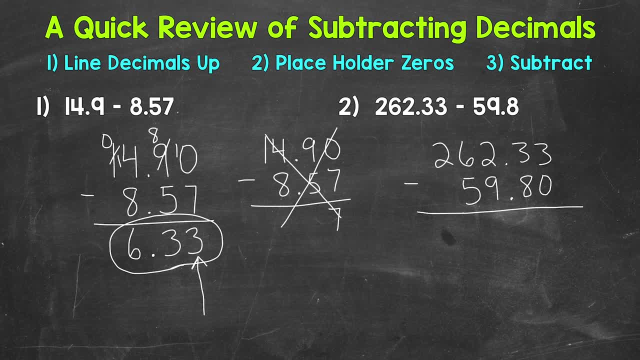 We can use a placeholder zero, so these both go to the hundredths, And now we are able to. So we will start with the hundredths. 3 minus 0 is 3.. The tenths place 3 minus 8,. well, we need to borrow. 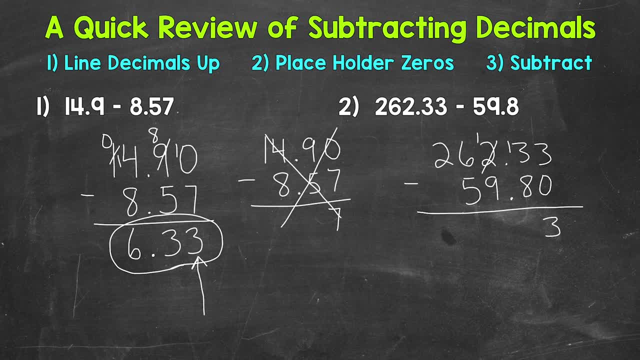 So borrow from the 2,, that's a 1, and we have a 13. So 13 minus 8 is 5.. We can bring our decimal straight down into our answer. And now we have the ones place. So 1 minus 9, we need to borrow. 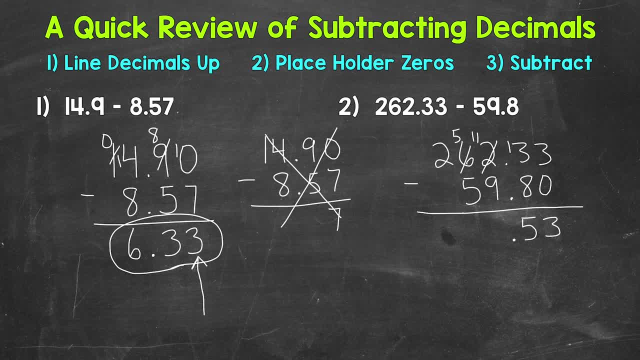 So we will borrow from the 6. And we have 11 minus 9,, which is 2.. Then, for the tens place, we have 5 minus 5,, which is 0. And then, lastly, we have the hundreds place, where we have 2 minus nothing under it. 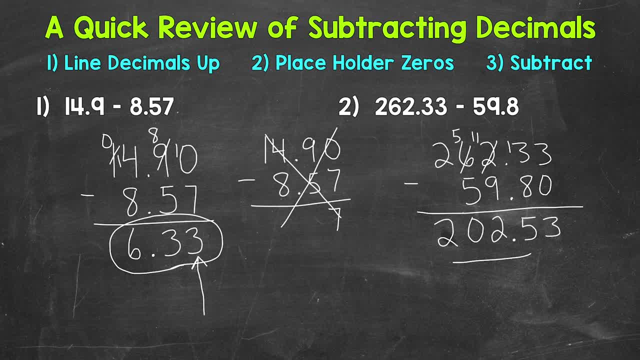 So it's just 2 minus 0, which is 2.. And our final answer 202 and 53 hundredths. So there you have it. There's a quick review of subtracting decimals. Line the decimals up. Use placeholder zeros if need be.